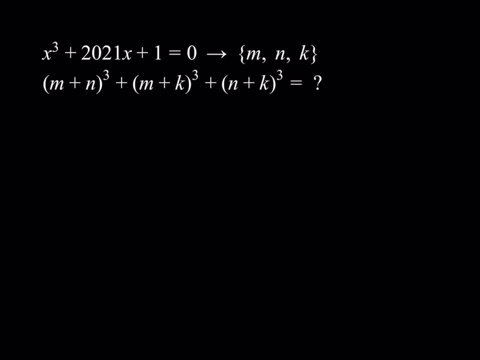 differently, And I'm going to present two solution methods here. So let's get started Now. the first thing I want you to notice is that this equation is missing the x squared term. Therefore, if you write your cubic as ax cubed plus bx squared plus cx plus d is equal to zero, we have b equals zero. 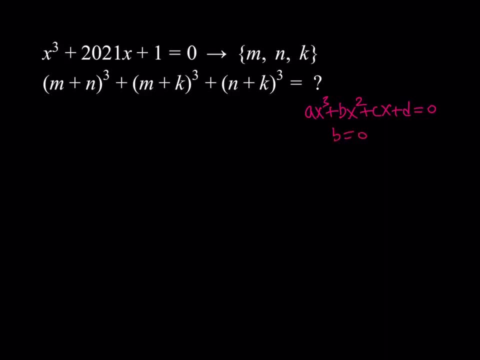 Awesome. Now what is that supposed to mean? Well, you know that in a cubic equation, x1 plus x2 plus x3 is equal to negative b over a, which is always true for any type of polynomial equation. right Cubic quartic quintic doesn't matter. So if b equals zero, that means the sum of the. 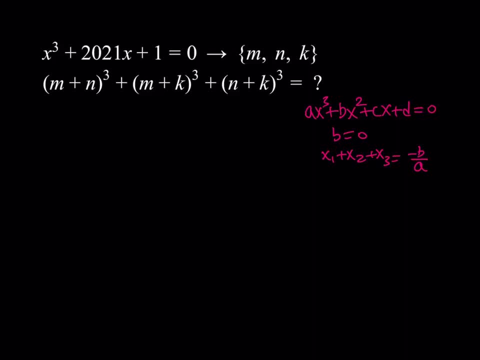 roots is also zero. So from here we get the important conclusion: m plus n plus k is equal to zero. So that's going to be our first relationship, Great Great. So you can see that the sum of the roots is also zero. So from here we get the important conclusion. 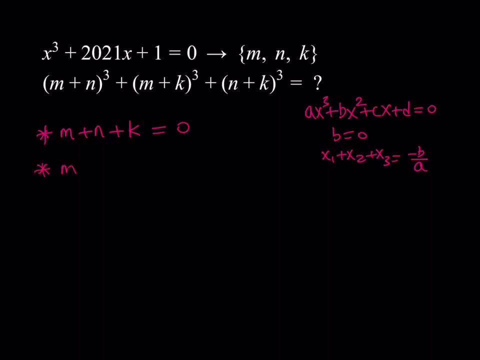 m plus n plus k is equal to zero. So that's going to be our first relationship, Great, Great. So what is my second one? Well, second one is going to be the two-way products: mn plus mk plus nk. Now, 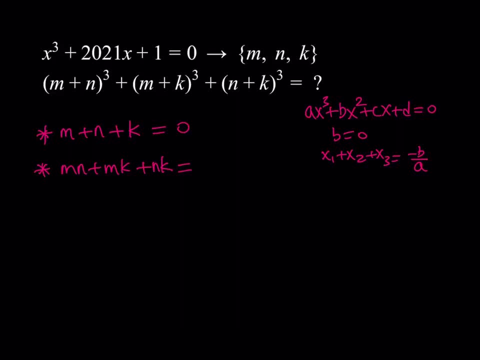 how do you find that? That's c over a? And in this case c is the coefficient of x, But it's not c over a, It is actually c over a. I mean, what am I talking about? It's positive c over a, So it kind. 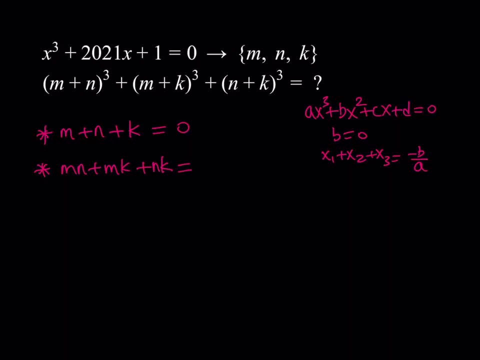 of goes like negative, positive, negative, positive. They're going to alternate. So this is c over a, And since a is one, this is just going to be 2021.. Cool, Okay, nice. What else do I know? 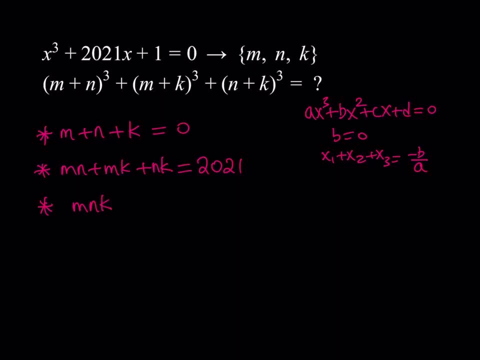 Well, the product which is going to be negative d over a in this case is going to be negative one. Cool, You can again look at that video for reference for Vieta's formulas. Now, what am I going to do with this? Well, I'm supposed to evaluate this expression and I'm going to be 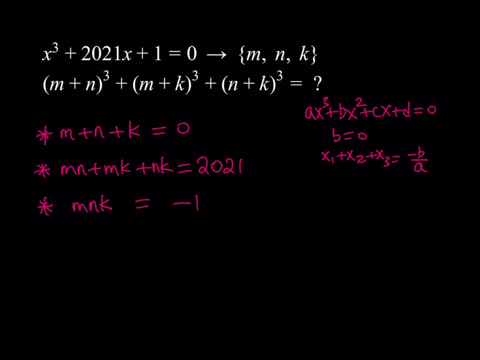 using these. So, like I said earlier, I'm going to present two methods. Here's the first solution method. First of all, notice that these expressions m plus n, m plus k and n plus k without the cubes. So I'm going to present two methods. Here's the first solution method, First of all. 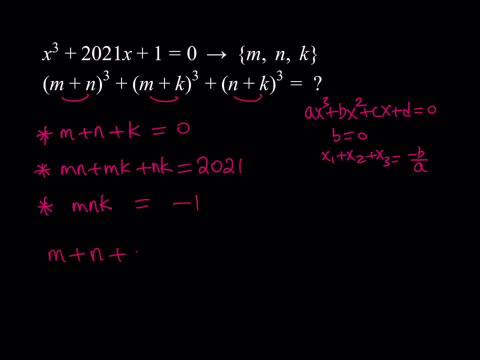 give us something interesting. If you add them, what do you get Without the cubes? of course, If you add them without the cubes, you get two times m plus n plus k, right? Well, we know that m plus n plus k is equal to zero. So this is also zero, because two times zero equals. 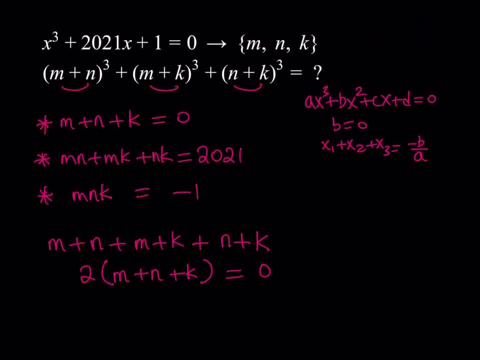 zero, right? What is that supposed to mean? Well, it is significant because we have a special expression for that. If a plus b plus c is equal to zero, then a cubed plus c is equal to zero. Okay, what am I talking about? Okay, let me write it down. Let me write it down. Here's the formula. 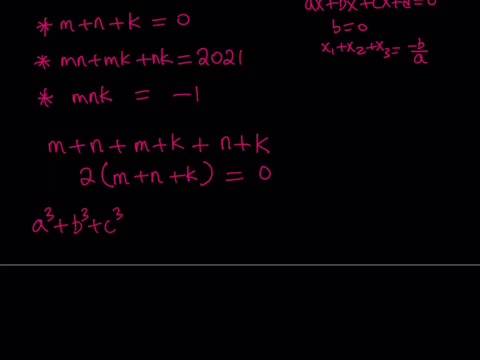 In other words, we can subtract this weird polynomial. And, to make matters worse, this polynomial is divisible by a plus b plus c. Would you believe that? Well, if you don't, you can kind of verify it. But yes, it is. So this polynomial is divisible by a plus b plus c, And 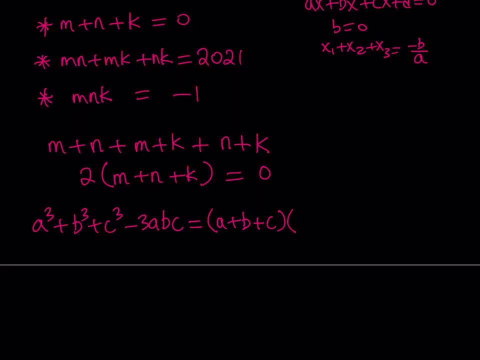 the other factor- and again, we've done this in another video, so you can also look at that too. Maybe I'll try to include that link as well- And the other factor is going to be a squared plus b. squared plus c. squared minus ab, minus ac. 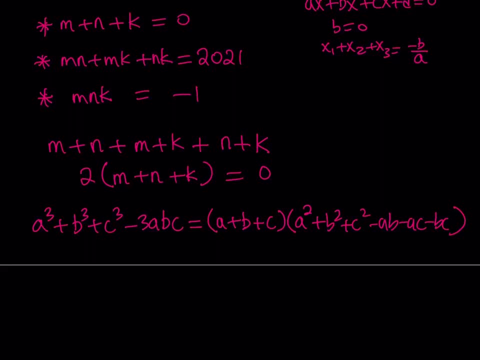 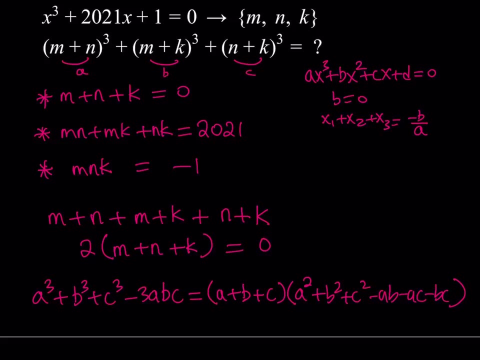 minus bc. Now, why is this significant? It is significant because if you call this a, if you call this b and if you call this c, we have that a plus b plus c is equal to zero. This is a plus b plus c, right? Well, if a plus b plus c is zero, that means this is zero. 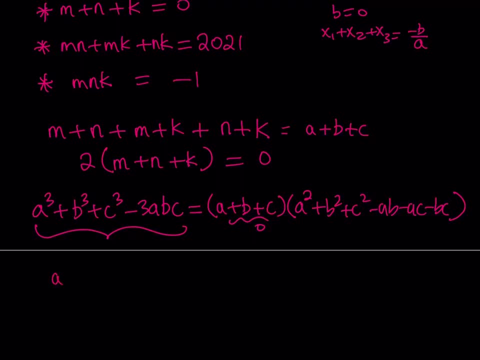 Therefore, this is also going to be zero, which means you have a cubed plus b cubed plus c cubed being equal to three abc. Nice, So what am I trying to find? Well, I'm trying to find a cubed plus b cubed plus c cubed. That's what I'm trying to. 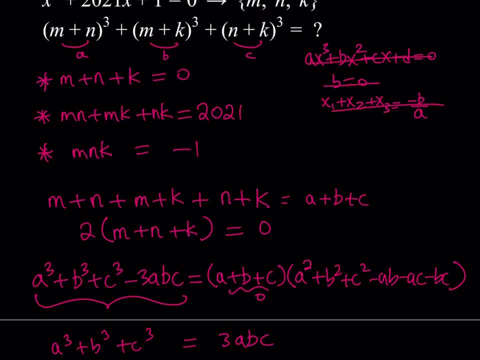 find. Well, by the way, this a and that a are different things, So don't worry about that. Okay, let's erase this one. So that's a different a. So well, what is abc? Well, abc is not the mnk. 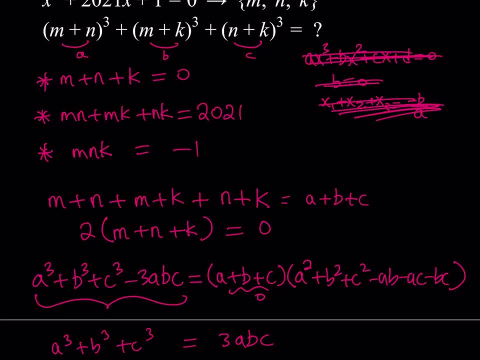 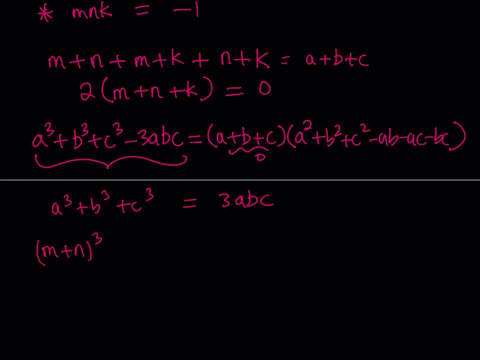 of course It is the product of all these quantities without the cubes. So I'm trying for this. And so, in other words, m plus n cubed plus m plus k cubed plus n plus k cubed is equal to three times m plus n, times m plus k, times n plus k. Now you might be asking like: 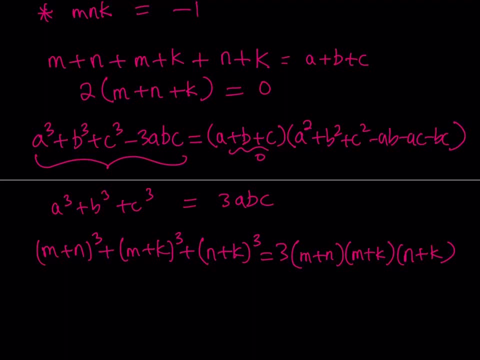 what is so significant about this? We were trying to find this, but now you complicated things. Do we know how to find this? Well, you can go ahead and distribute, And obviously this is better than the other one, because that's a sum of cubes. This is kind of like a product a lot easier to handle. 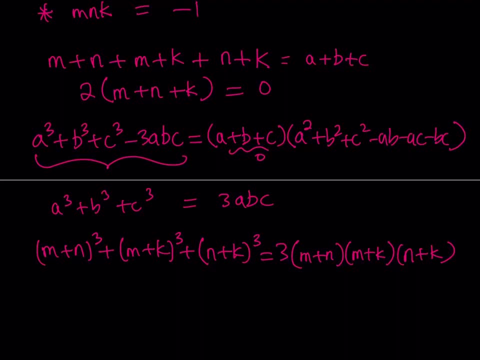 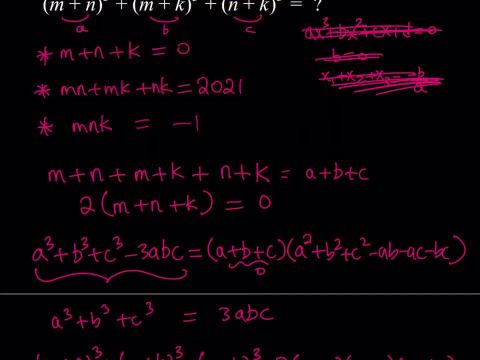 But again, we're going to make it nicer. This is not nice enough And I'm going to make it nicer How We're going to use the relationship again And it keeps popping up right. So it's a super important relationship that m plus n plus k is equal to zero. This is super duper important. Why? 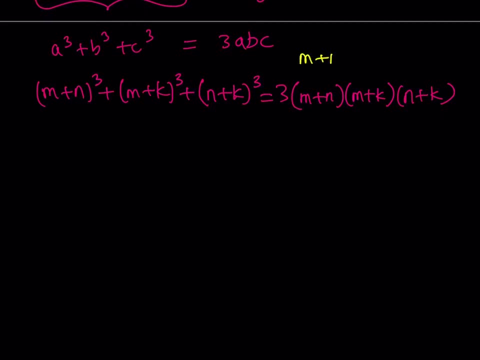 Because, if you look at this, if I know that m plus n plus k is equal to zero, that allows me to write each one of these in terms of the third one, For example, m plus n can be written as negative k. m plus k can be written as negative n. n plus k can be written as negative m. So what? 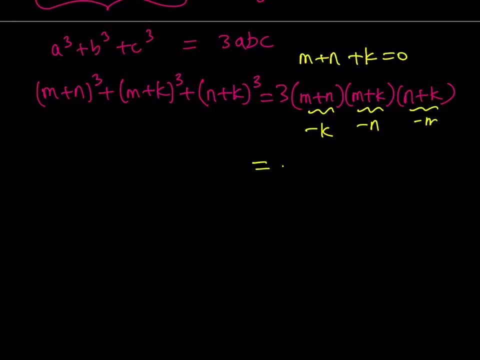 is that supposed to mean? What I'm trying to find, then, is equal to negative, because I'm multiplying three negatives, that makes a negative negative three m n k. Well, do I know m n k? Yes, I do Remember. at the beginning we calculated it, So we do have. 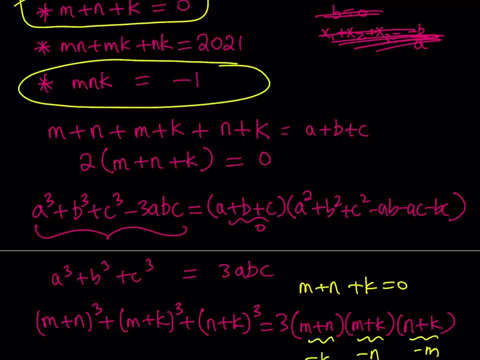 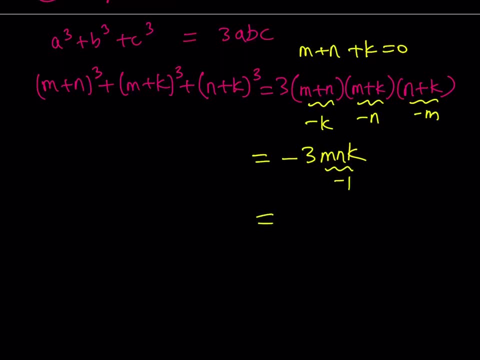 that relationship And I told you that we were going to use it. Now we're using it. m n k is equal to negative one. from Vieta's formulas, If this is negative one, negative three times negative one is positive three. So what I was looking for, the expression, this gigantic expression, here. 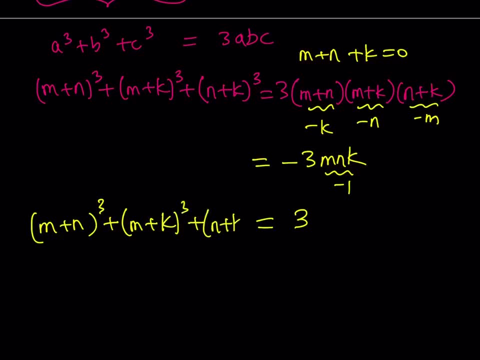 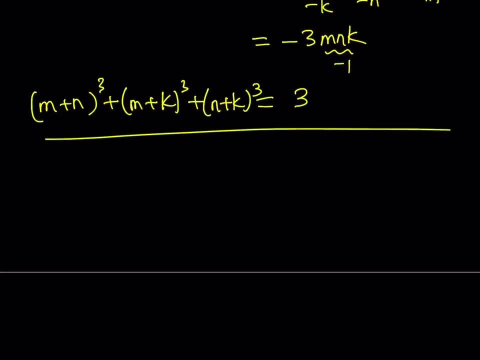 the sum of three cubes is equal to three. That concludes the first solution method. Okay, so the answer is three. Now I'm going to present the second method And then you can decide. please let me know in the comment section which method you think is better or? 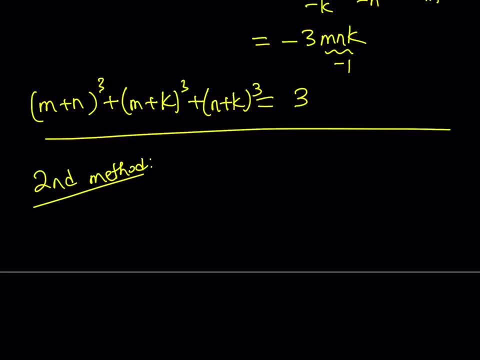 which method you like better. Of course, everybody has their own preferences And I will also share mine, Okay. second method involves a little different strategy. Well, I can't say completely different, But let's start with what we're trying to find. this one, Okay. so I'm trying to. 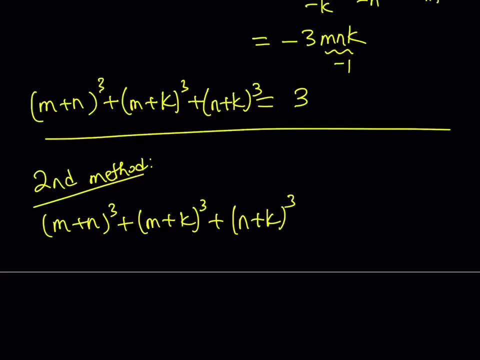 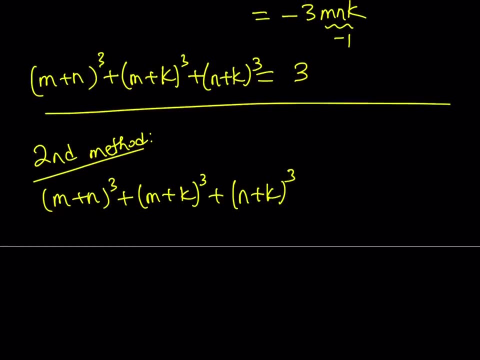 simplify this or find the answer Again. we're going to go back to this idea here And we're using it at the beginning, In other words: right, it's kind of easier. I don't know. m plus n is equal to negative k. this is equal to negative n, So let's go ahead and write that negative k. 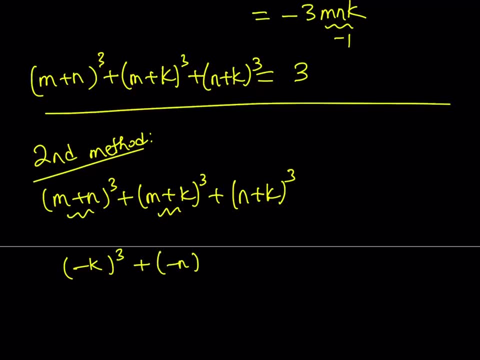 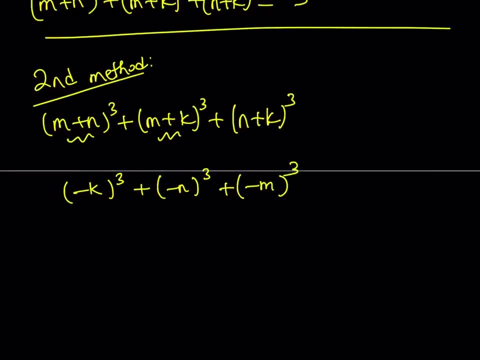 cubed plus negative n cubed plus negative m cubed. Great. Now, if you cube a negative number, you get a negative answer. So they're all going to be like negative k cubed, negative n cubed, negative m cubed, And obviously we can put a negative sign on the outside and write them in. 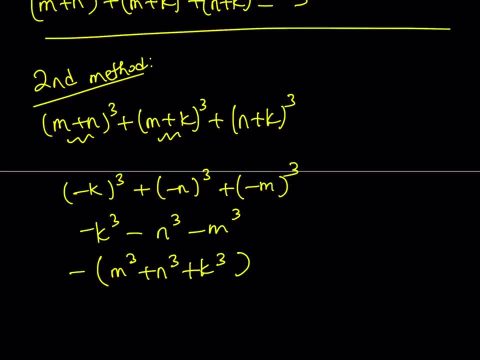 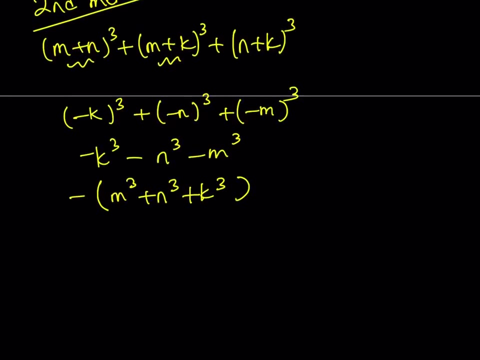 kind of alphabetical order, ish right, something like this And you're going to get that. So what I'm trying to find is actually equivalent to this. this is nicer because it's not like a two way addition cubed, it's just a singles cubed sort of. So this one is a little easier to find. But 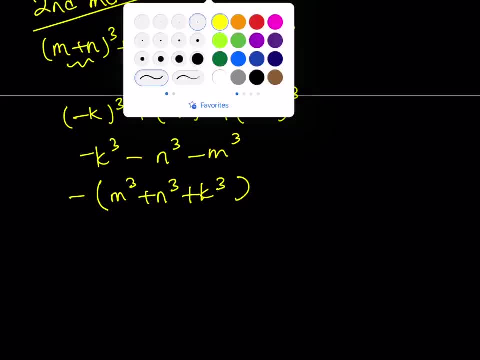 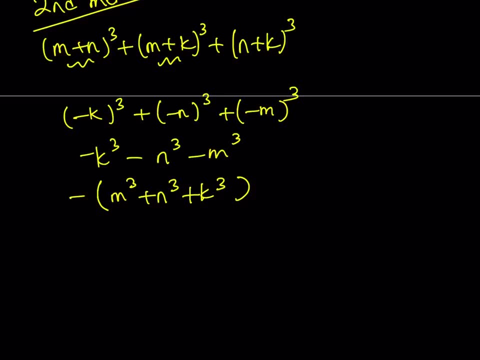 in order to be able to find that I'm going to use a little algebra, which is kind of fun. I mean, the second method is going to take longer, But it's a there's a different flavor to it. Okay, cool, Let's take a look Now. what am I going to? 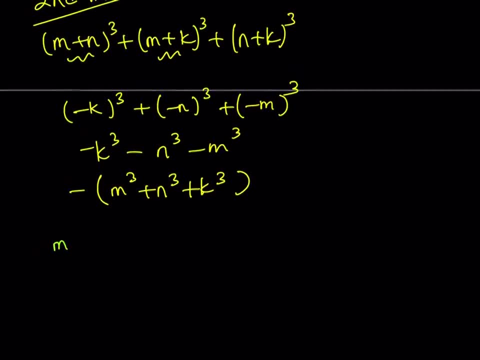 do In order to be able to get the sum of the two cubes. obviously- and I think that should be kind of obvious- I'm going to go ahead because we don't have a formula. Okay, so we have a formula for a cubed plus b cubed, But we don't have necessarily have a formula. Well, we kind of do. 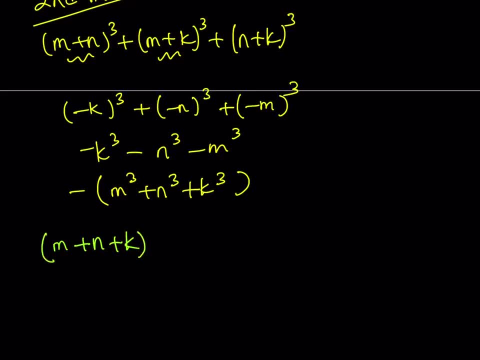 but whatever, Let's just do it. Okay, this is what I was trying to do. Let's cube this expression. Okay, what do you get when you cube it? Well, I can treat this as a single entity, or single entity whatever, or single expression, and then do it that way, kind of like. 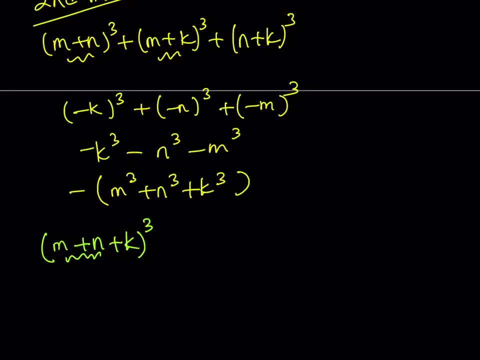 a plus k cubed or z plus k cubed, Make sense. Okay, it's gonna look like this: m plus n is going to be my first term, cubed plus three, Again using the binomial theorem. I'm just gonna. 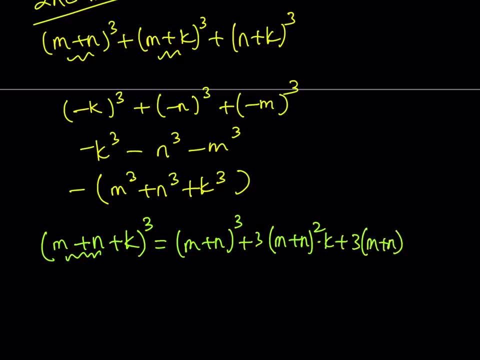 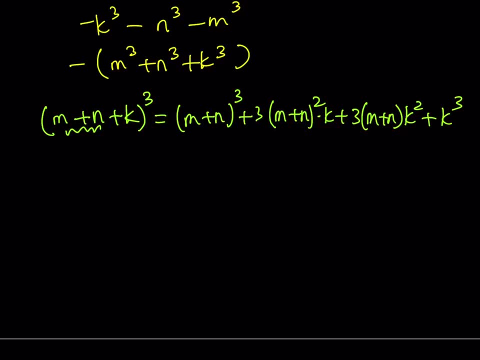 you know, write the formula, mix it up, Okay, like this, and then finally k cubed, Cool. Of course, this requires a little bit of expansion here, And if you do expand it, you're gonna get something nice. Well, it's not gonna be super nice, but I can't guarantee that. 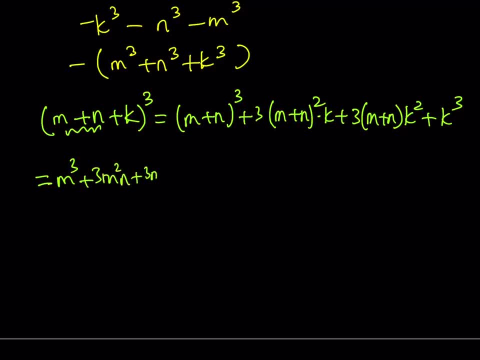 right, Three m squared n plus three m n squared. I'm probably gonna need a little bit more space. I feel like Let me start over here all the way here, So kind of like let's see m cubed plus. 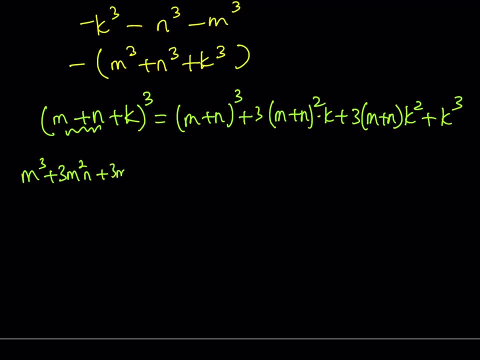 three m squared n plus three m n squared plus n cubed. And then notice that when you expand this it's gonna look like m squared plus two m n plus n squared. And you're gonna multiply it by by three k. so consider that. So it's gonna look like three k m squared plus six m n k, Kind of. 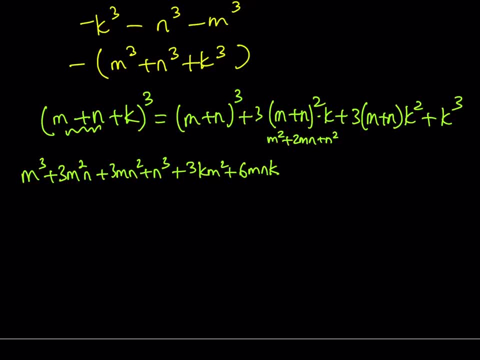 looks like square kilometers, right, Okay. And then multiply three k. by that you're gonna get three k n squared. When you distribute that, you're gonna get three k squared m. three k squared m plus three k squared n, And then, finally, you're gonna be getting k cubed. Okay, that's kind of. 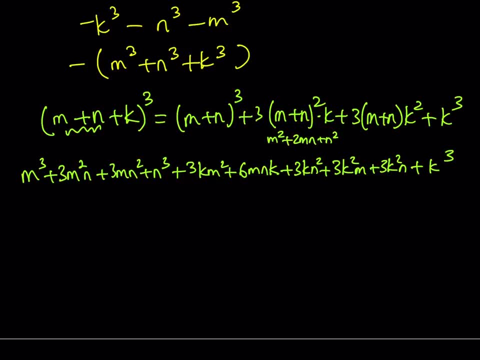 like a mouthful right, But we're gonna arrange these terms And, trust me, it's going to simplify, it's going to be really nice. I'll take m cubed plus n cubed plus k cubed, because that's what I'm trying to find. Remember, our expression depends on this. 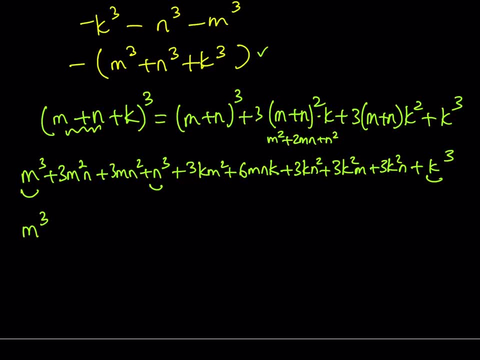 but just the negative of it. So once I find the answer from here- m cubed plus n cubed plus k cubed- I'm just going to negate it. That's going to be the answer. Cool, So that's the first part. 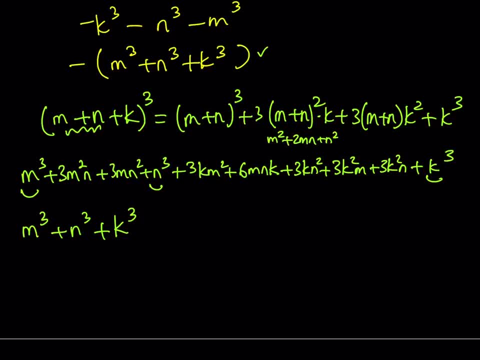 The second part. I gotta be smart and put these together in a meaningful way. How Well? I gotta take these two together, but factor out three m? n and write it like this, because you'll see in a little bit Okay. 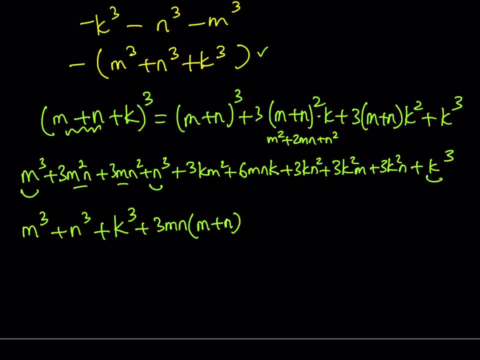 And then the next thing you're gonna look at should be something like these two, because again they're kind of friends, good friends, whatever- Three k m times m plus k- You get the idea, hopefully, from symmetry- And then these two guys are gonna go next and then that's gonna be three. 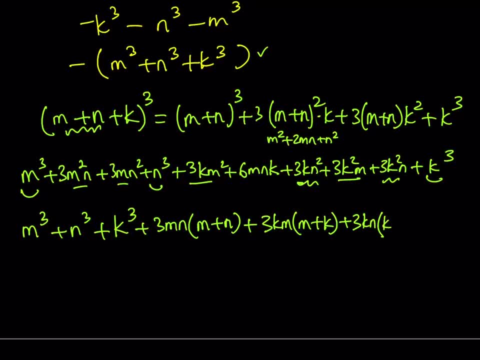 k n multiplied by k plus n, You get the pattern hopefully. But we still have a leftover, and that is the glorious term, which is six m n k. It's kind of like by itself, right. So this is basically a formula kind of for m plus n plus k cubed. 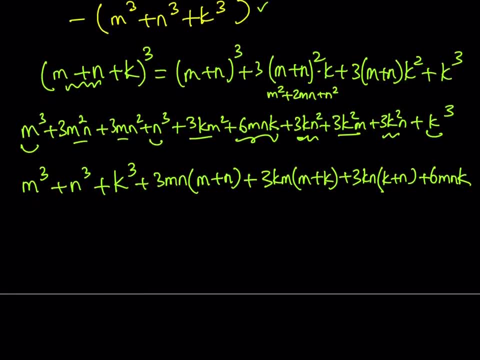 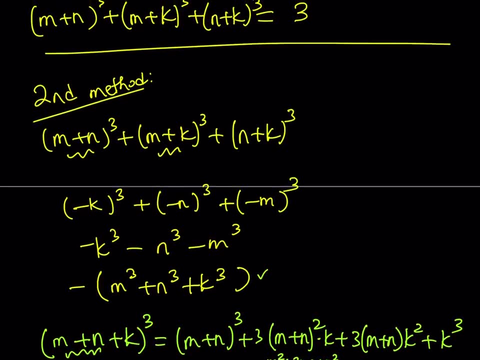 All right, But I'm trying to find the sum of the cubes. Well, how does this help me? Again, we're gonna go back to the same idea. Since m plus n plus k is equal to zero, m plus n can be written just like here: negative k, and so on and so forth. 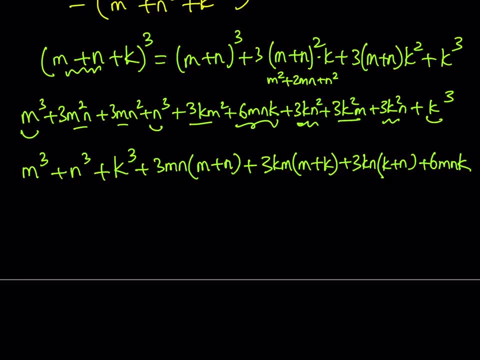 so I can replace m plus n with negative k. I can replace this with negative n. I can replace this with negative m. Beautiful, Awesome, And you're gonna see in a little bit why this is so awesome. because it's awesome. Okay, Cool. This is gonna give me negative three m n k minus three m n k. 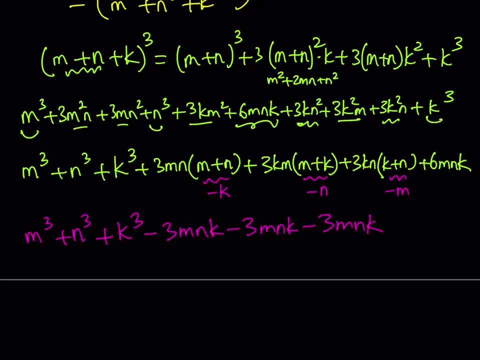 minus three m n k. You see how awesome that is. Plus three, I mean plus six m n k. Now notice that I have a little bit of a problem here. I have a little bit of a problem here. I have a. 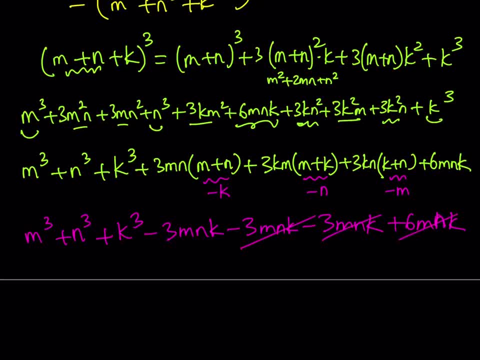 problem here. Notice that these two guys will cancel this out. We're gonna end up with this guy over here. Wow, That's interesting. But what was this whole thing? equal to right. Well, I was trying to expand this, right? Oh, this is where it comes from, Nice, But m plus n plus k. 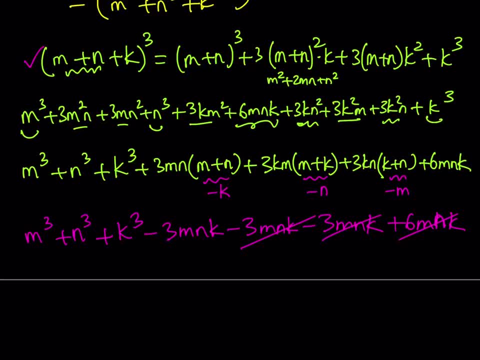 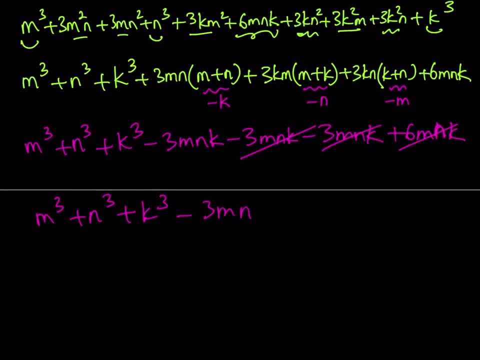 is equal to zero. So this is equal to zero. Wow, That's interesting, And I was trying to find something like this, right. So in other words? in other words, this guy is equal to zero because it's equal to m plus n plus k quantity cubed. Well, what is that supposed to mean? If you isolate? 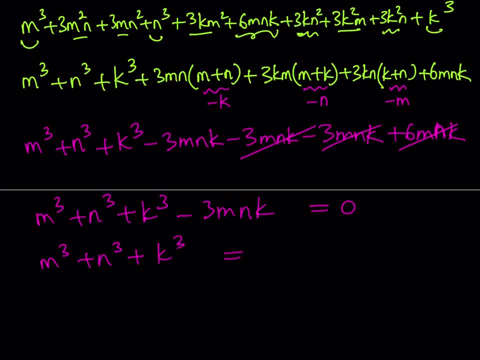 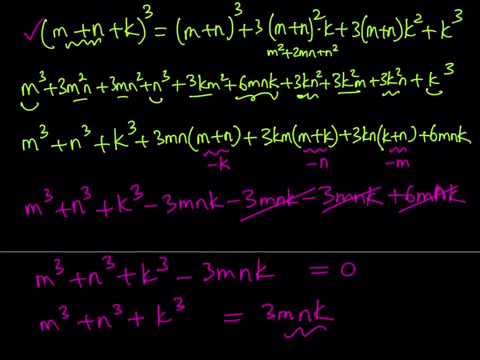 this sum, then it's going to equal three m n k, And we know that m n k is equal to. we found it before, right, Didn't we? It's equal to negative one. Awesome, So this is equal to negative one. 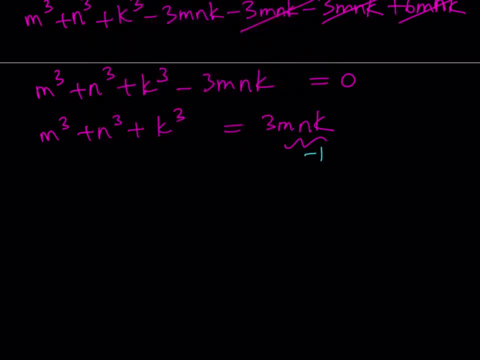 What is that supposed to mean? Well, if this is negative one, then this is equal to negative three. But if you remember, if you remember m plus n cubed plus m plus k cubed plus n plus k cubed was what I was trying to find And it was equal to. we proved that it was. 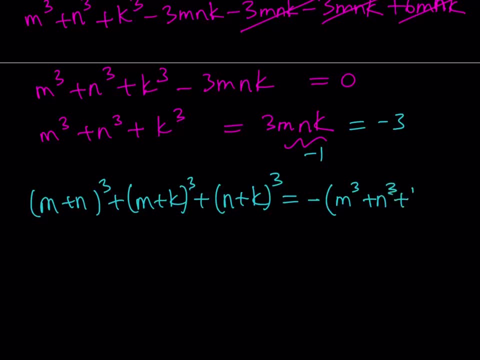 equal to the opposite of this expression. Now, if this expression, the sum of cubes, is equal to negative three, if you negate it one more time, you're going to get three. So the three is going to be the answer. And this concludes the second solution method, which brings us to the end of.